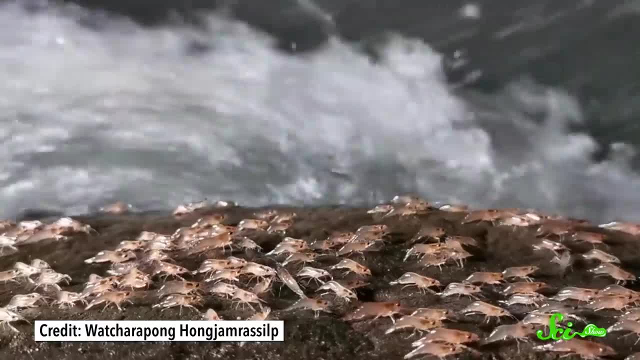 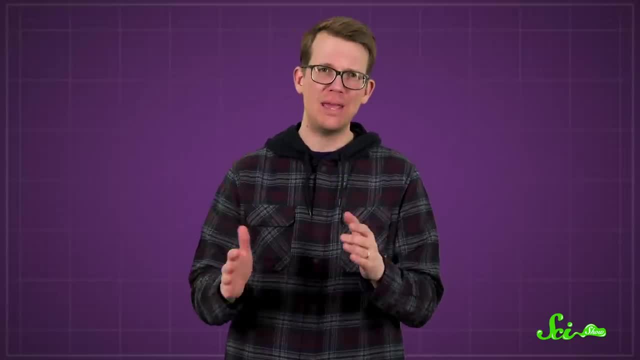 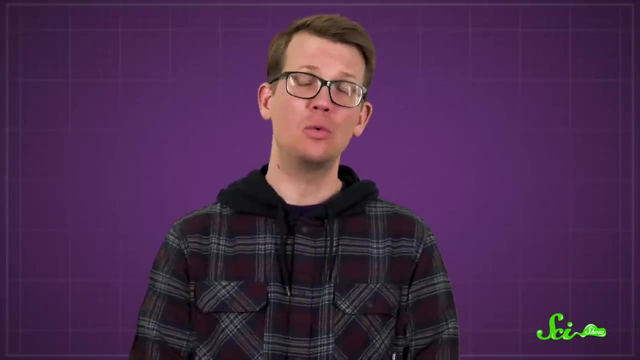 All night long, streams of tiny shrimp march out of the water and parade along the river's edge, And they have to have a really good reason to take a risk this big. But until recently, no one knew why they did it. Now, if you're not familiar with shrimp, walking is a weird way for them to get around. 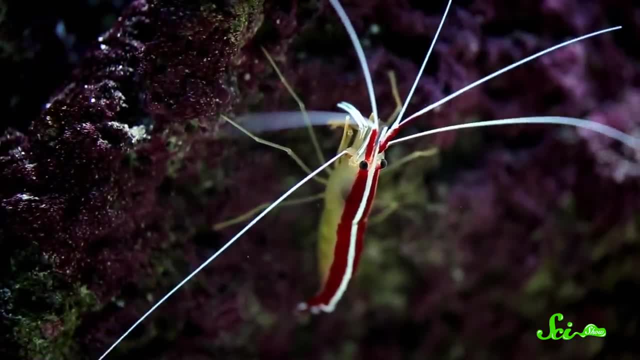 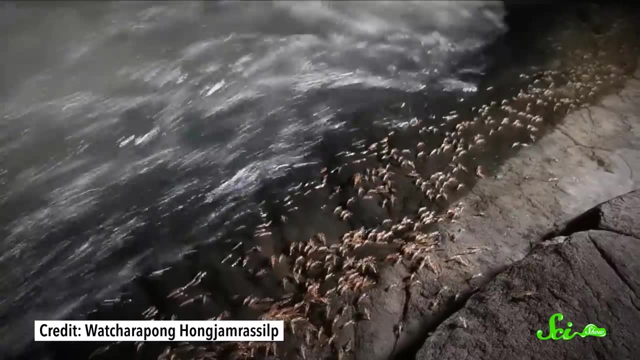 Shrimp are aquatic animals. Like they have gills, and if they dry out they die. Plus, there's a slew of predators on land waiting to eat them. Yet here, these less-than-one-centimeter-long shrimps are leaving the water for ten minutes. 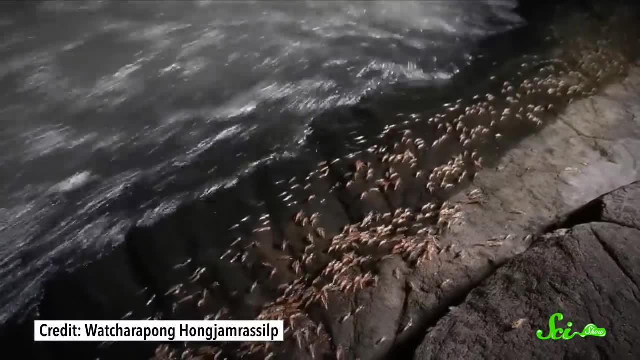 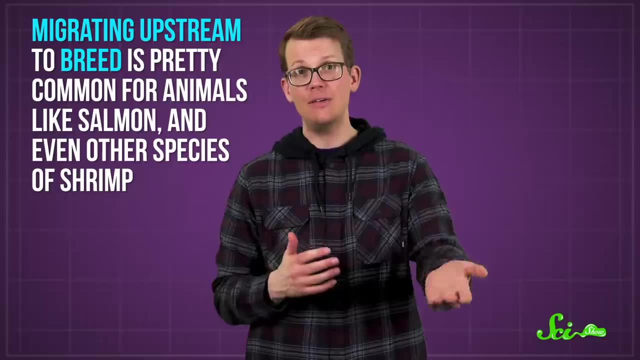 or more, and crawling some twenty meters onto land. The local lore was that it had to do with breeding. Migrating upstream to breed is pretty common for animals like salmon and even other species of shrimp, so it's a pretty good guess. 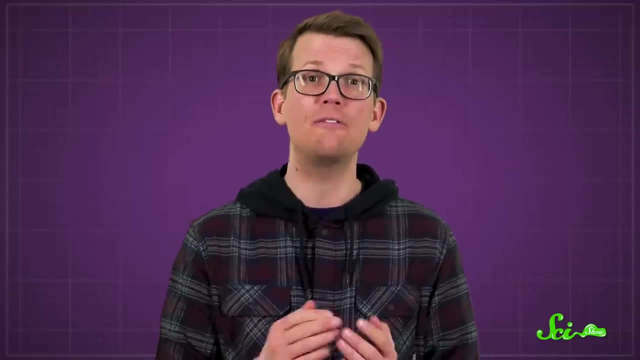 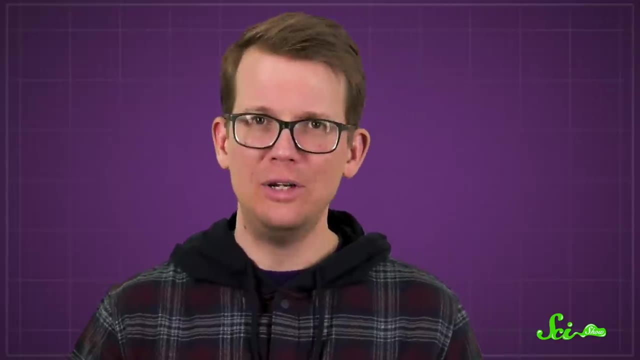 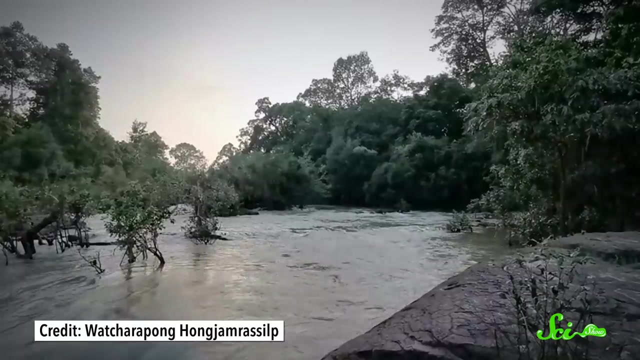 But when scientists systematically studied the parading shrimp, they found that they were almost all juveniles. That meant they were too young to mate or spawn. Instead, the reason was much simpler and cuter: It's to avoid strong currents. Researchers realized two of the most reliable places to see these shrimp parades. 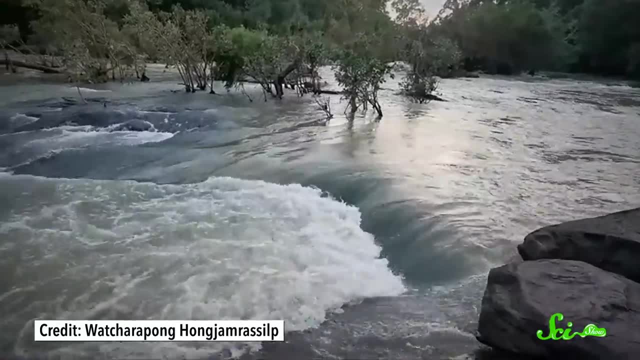 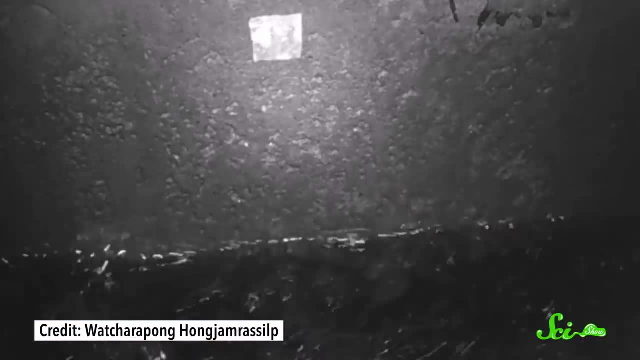 were next to a set of rapids and a small artificial dam. So for a 2020 article, they tested this idea in the lab. They set up tanks where they could vary the current And, lo and behold, the smaller shrimp got out whenever the current was too strong. while the larger ones could still swim. That's why, in the wild, these shrimp that walk on land are so teeny. Bigger ones are also going upstream, but they swim instead. What we don't know for sure is why they're so keen to go up the river. 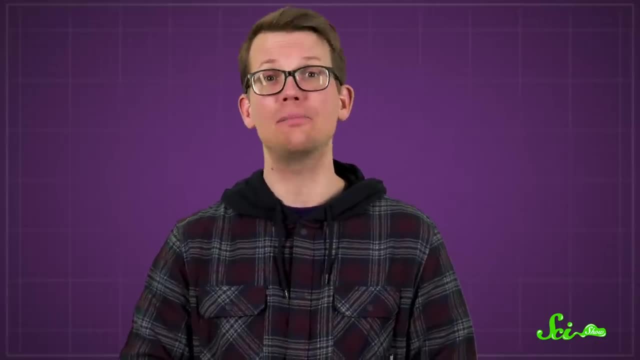 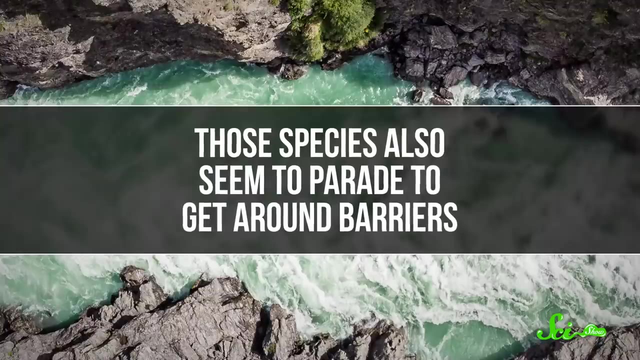 For clues, we had to look at other shrimp. They're not the only shrimp that parade, because, yes, apparently other species do this as well, including ones in India, Australia and the Americas. Those species also seem to parade to get around barriers. 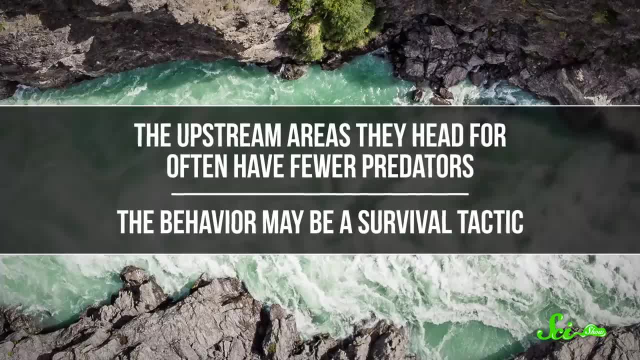 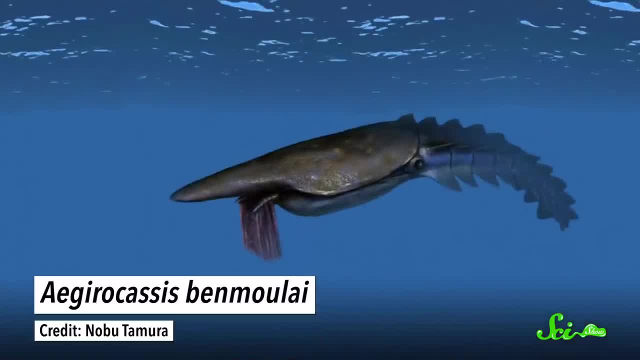 And the upstream areas they head for often have fewer predators, so the behavior may be a survival tactic. It may also shed light on how shrimp colonized freshwater habitats in the first place. Their ancestors most likely came from the ocean, so gaining the ability to walk around barriers. 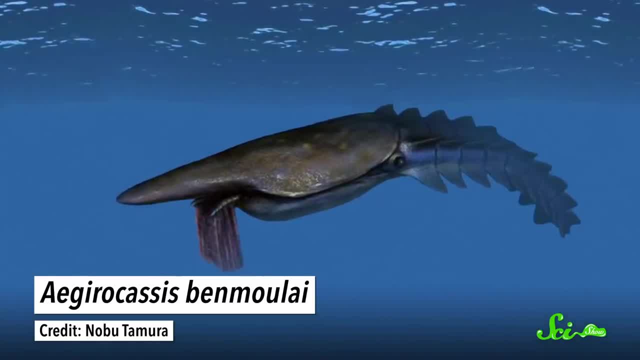 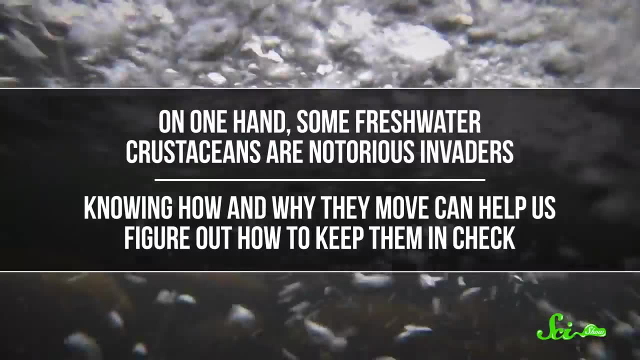 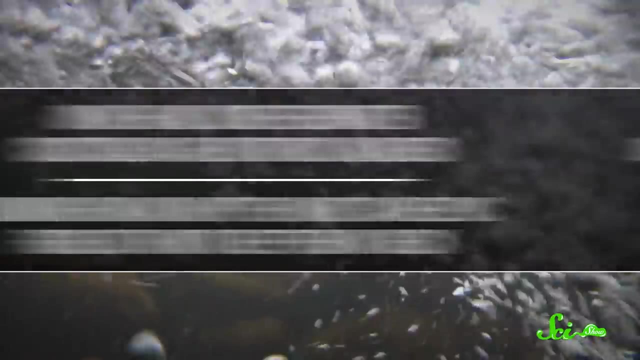 may have been a crucial part of the move into resource-rich freshwater habitats, But, more practically, further research on shrimp parades could help us take better care of them and their habitats. On one hand, some freshwater crustaceans are notorious invaders, so knowing how and why they move can help us figure out how to keep them in check.